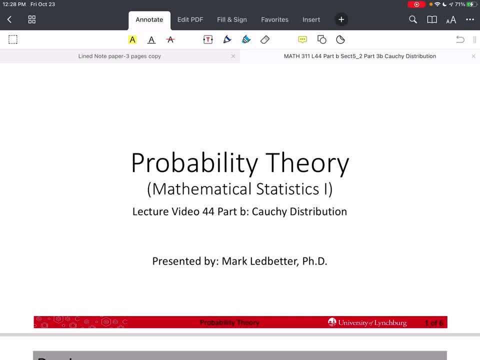 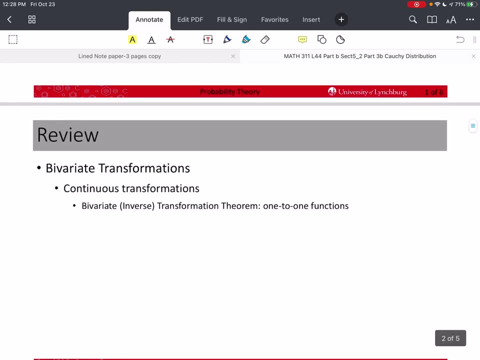 Welcome back to our series on probability theory. I'm Mark Ledbetter and this is lecture video 44. We are doing part B and we're going to cover the Cauchy distribution. We've been talking about bivariate transforms, transformations using one-to-one functions. 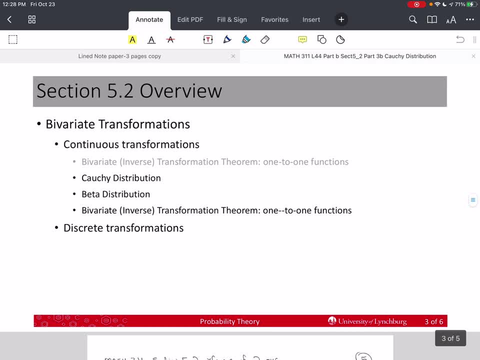 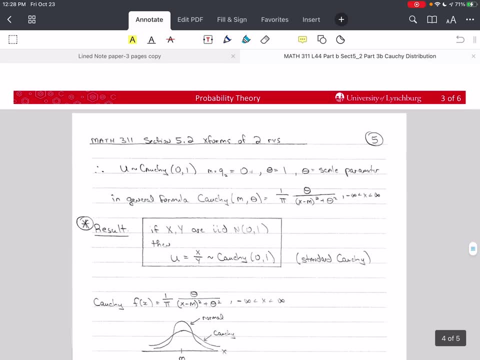 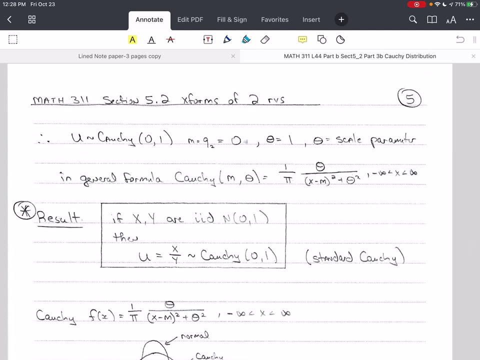 and we're going to need some new or some additional distributions for some of the examples we're going to work. So the first one is the Cauchy distribution And the Cauchy distribution. we last time we found out that the ratio of two normal, standard normal distributions- 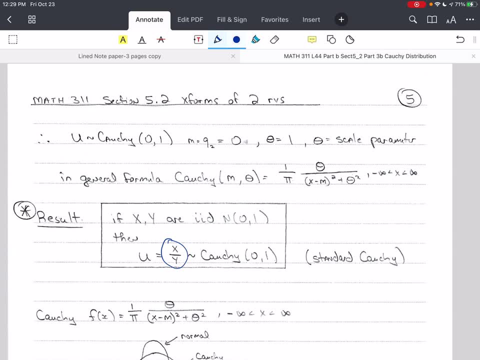 so the random variables that are distributed with a standard, normal distribution, that ratio is a standard Cauchy, Cauchy: 0, 1.. So what does the 0 stand for? The 0 is for the median, not mean, but median or Q2.. 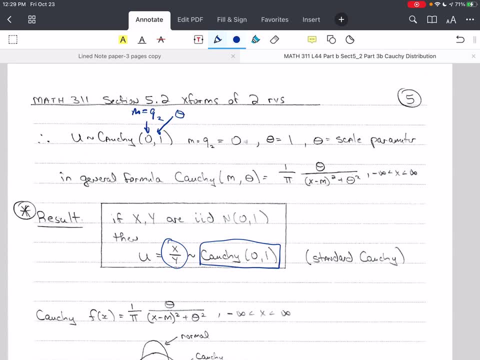 And the 1 here is theta, which is a scale parameter, how wide or narrow the distribution is. So we have a general Cauchy formula which is a little more complex but not much, And we've given that PDF here. 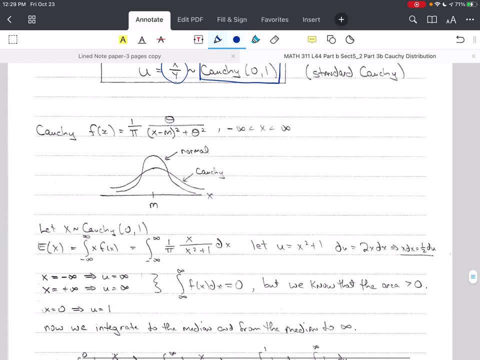 Okay, And we're going to learn a little bit more about the Cauchy distribution. So first, if you look, it's going to be symmetric about the median M, Okay, And the Cauchy is going to have a lower peak and thicker or higher tails than the normal distribution. 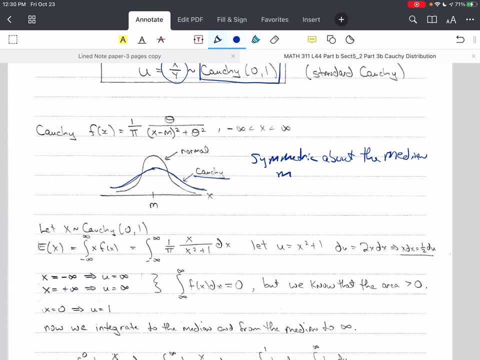 The normal distribution will have a higher peak in this sense. So we're going to use the standard Cauchy, because if it doesn't exist for that, it probably doesn't exist for or it doesn't exist for any of them. And this is the easiest or least complex of the Cauchy distributions. 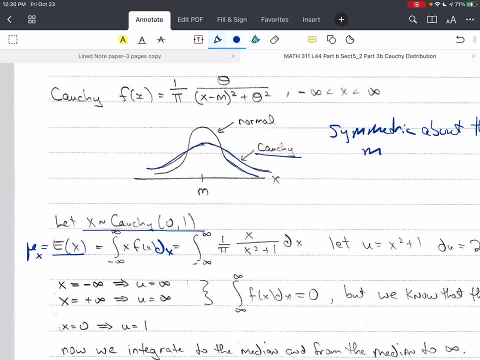 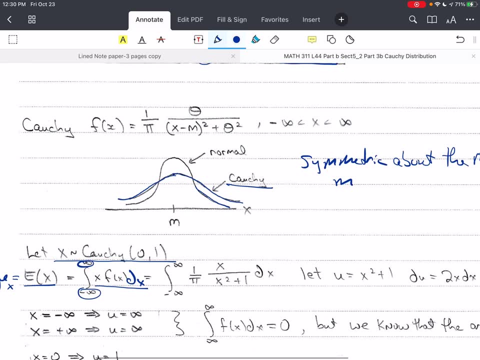 So the mean or expected value is: is x times f of x, dx, and integrated from negative infinity to positive infinity. Well, it turns out that x really is from negative infinity to positive infinity for the Cauchy. So the support of x is the entire real numbers or range of real numbers. 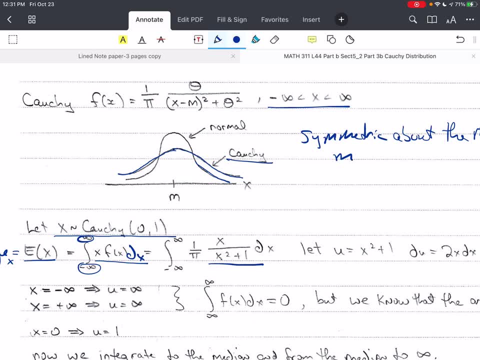 And so we plug in for the standard Cauchy and then x. So we have x times 1 over x squared, plus 1 times 1 over pi. Now, in order to integrate this, we're going to make a u substitution. 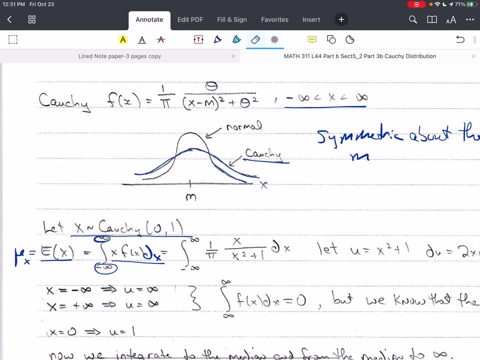 But before we get there, let's look at our limits of integration. So if I let x be negative infinity, then u becomes positive infinity. Okay, So I do need this u substitution right now. So x squared plus 1.. And so if infinity x is negative infinity, we square that positive infinity plus 1 infinity. 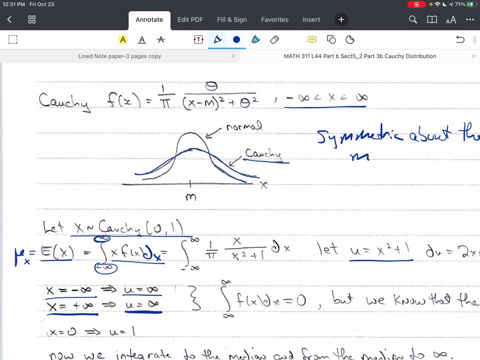 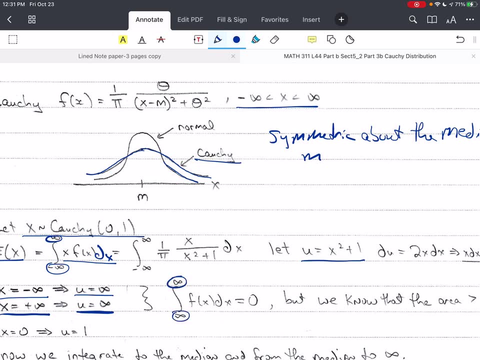 If x is positive infinity, same thing. We get positive infinity. Well, this creates a problem because now I would be integrating from infinity to infinity And that would give me an integral of 0. But we know that there is area we can see just looking at the curve. 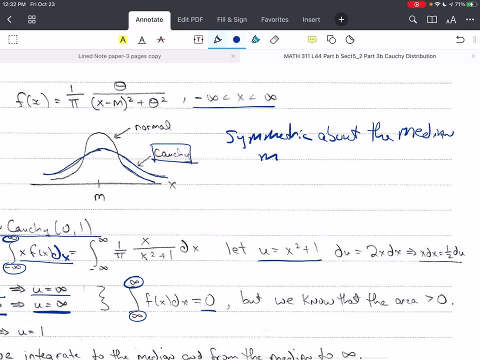 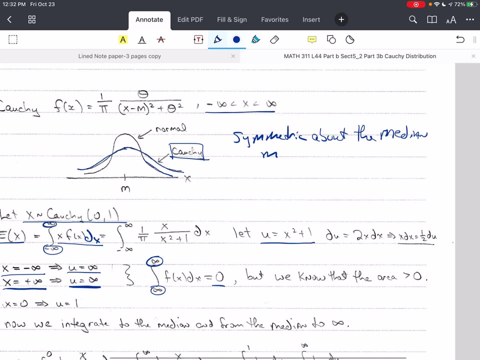 There is area under this curve. In fact it's the area under the curve itself is 1.. So multiplying that by x should give us a positive or a non-negative or non-zero answer for the integral of x. So we're going to integrate that integral. 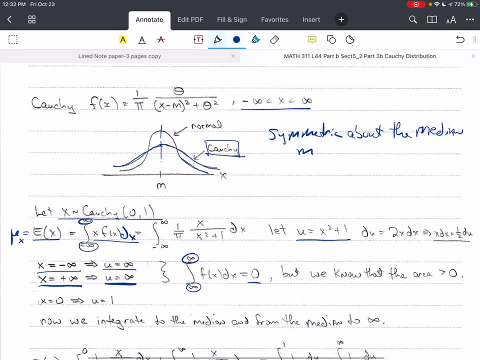 So we're going to integrate that integral. So, since it's symmetric about the median, not the mean, the median, and in this case m, is 0 for the standard Cauchy. so we're going to integrate from negative infinity up to. 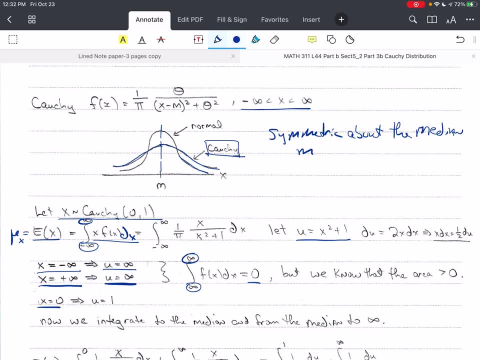 the median and then from the median up to infinity, Break it up into two parts, and that's perfectly acceptable to do So. let's look at the value of u when x is 0.. When x is 0, u becomes 1.. 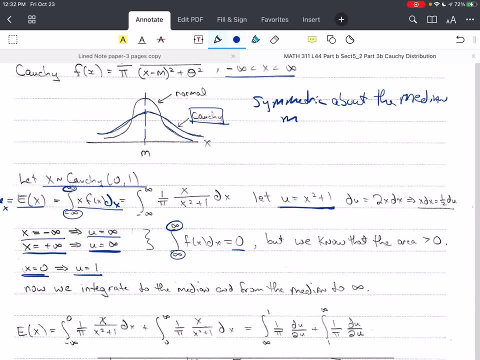 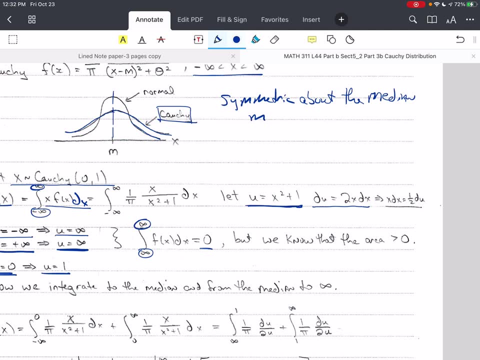 Okay, Okay, Okay. So now we're going to do the du and find out that it's 2x dx and then solving for x times dx, since that's what we have here. we see that that's 1 half du. 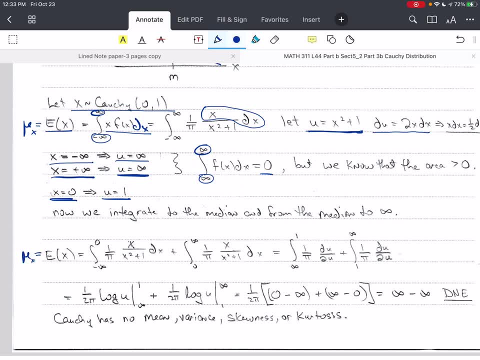 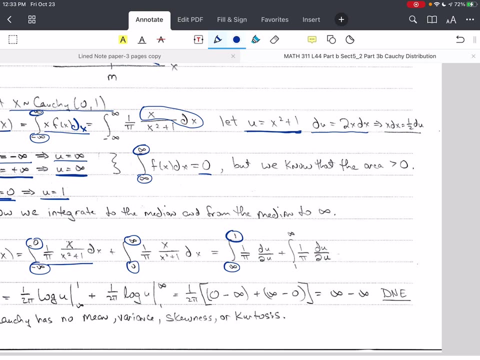 And so our mean, or e of x is the integral from negative infinity to positive infinity of our expression, plus from 0 to infinity, though this is under x, so when we make the substitution for u, it goes from infinity to 1.. 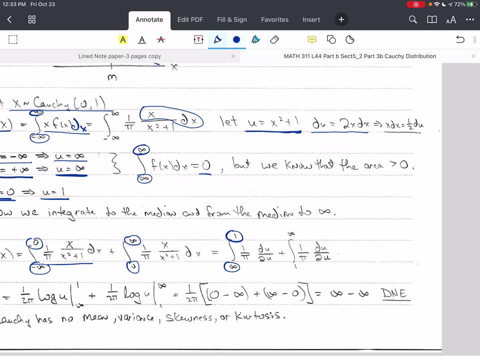 Do not change that. unless you're going to change the sign, It has to be from infinity down to negative 1 in this case. So we could change the signs- but I'm not going to- and make this a negative and that a positive and then you'd think it was 0, but it's not. 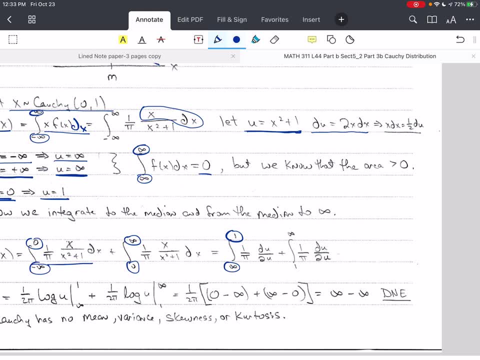 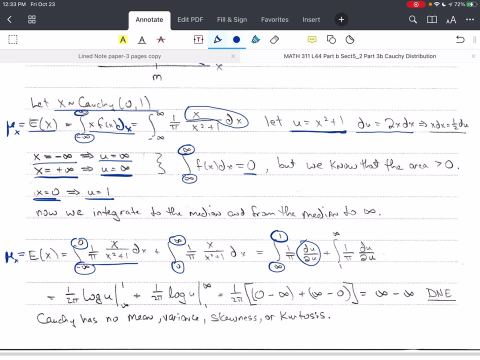 We have to be very careful with what we do here and when we end up with 1 over pi, du over 2u, and so the integral of 1 over u is natural log of u, And for statistics we use just log, because it's really the only log we use commonly. 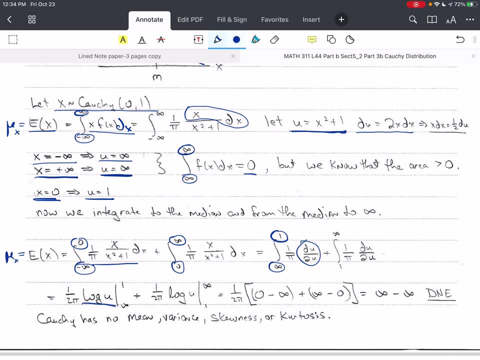 So we know that when we're statisticians and we see log u, that means the natural log of u. Okay, So we have this expression from infinity to 1, and then this expression from 1 to infinity and we see that we have 1 over 2 pi. 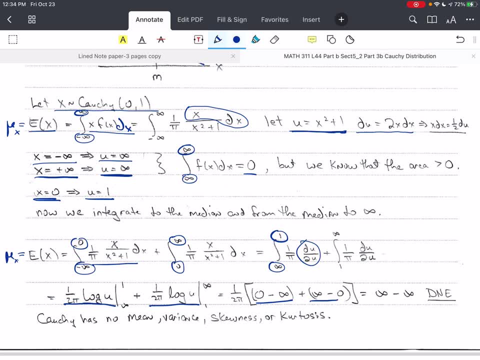 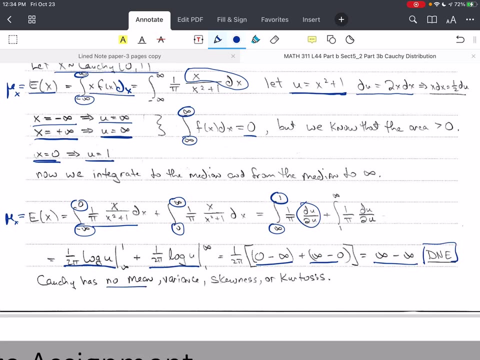 Negative infinity plus positive infinity, and that tells us that we can't evaluate this because infinity minus infinity is indeterminate, and it shows us that this does not exist. Okay, So there is no mean, no variance, no skewness and no kurtosis for the Cauchy distribution. 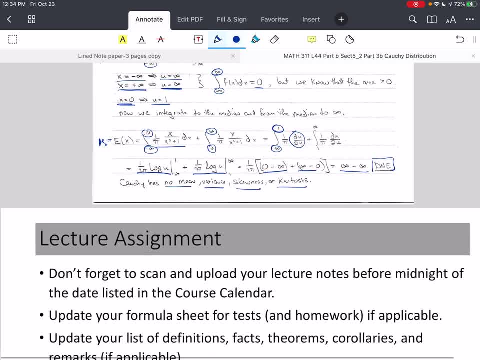 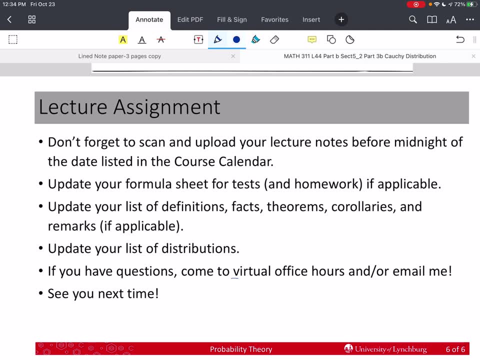 All right, So that's it for the Cauchy distribution. Please don't forget to scan and upload your lecture notes. You can do that by emailing me at the address or emailing me at the address. or emailing me at the address, I'll send you an email address and you can send me a picture of the problem, because 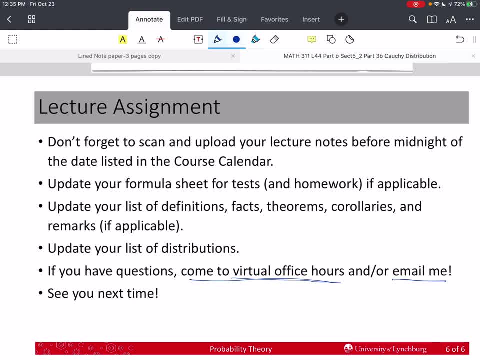 I may not have it handy- and a picture of your work so I can see how you're approaching the problem and that will allow me to help you quickly and efficiently through email. Please take care of yourself and we hope to see you next time.